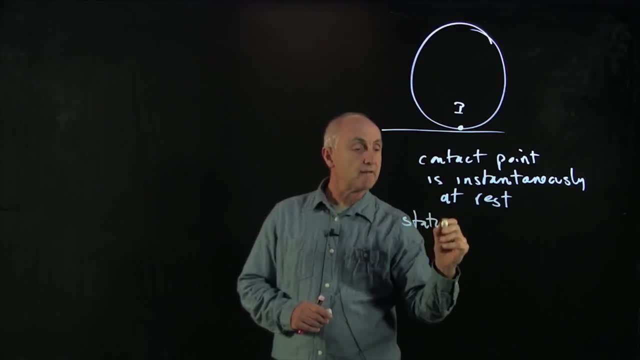 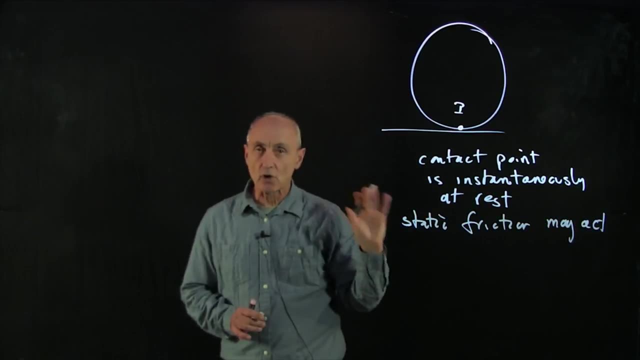 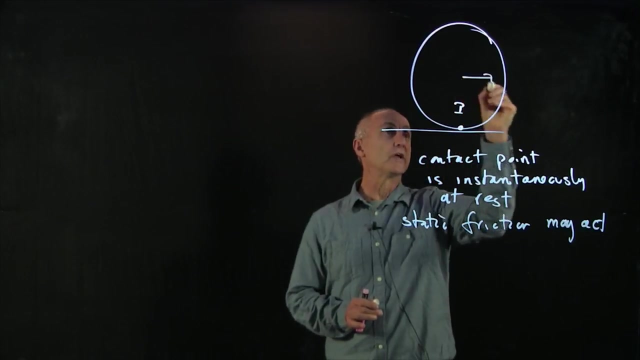 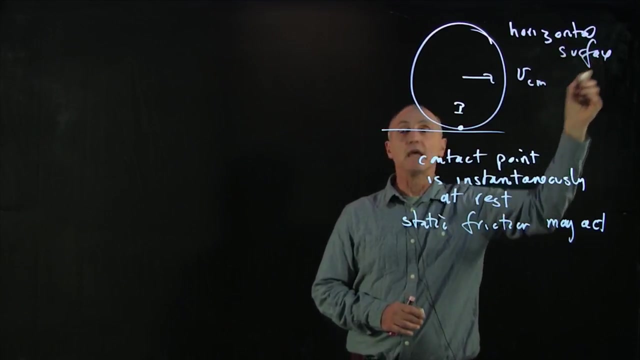 could be, static friction may act. However, static friction always depends on the circumstances. Now let's just consider two cases. Suppose here's a wheel VCM. This is a horizontal surface And in that case the static friction, if the wheel is rolling with a velocity v in. 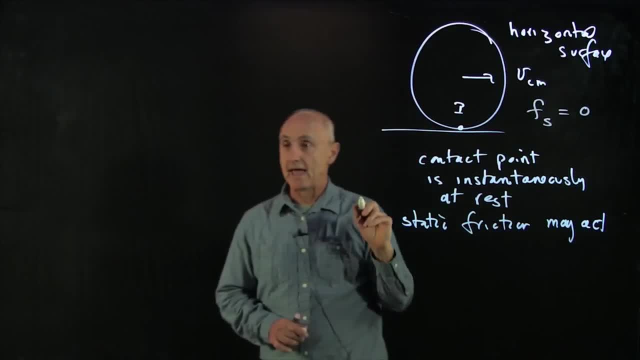 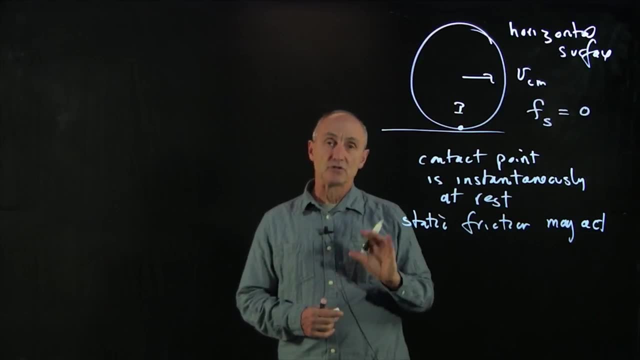 this case, f static is zero And because of that the wheel will roll without any friction, which is an idealization. There's other types of friction, called rolling resistance, air resistance, et cetera, which will slow the wheel down, But in a perfect hard wheel idealized. 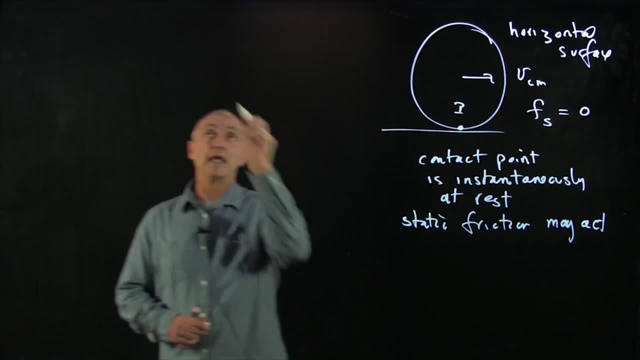 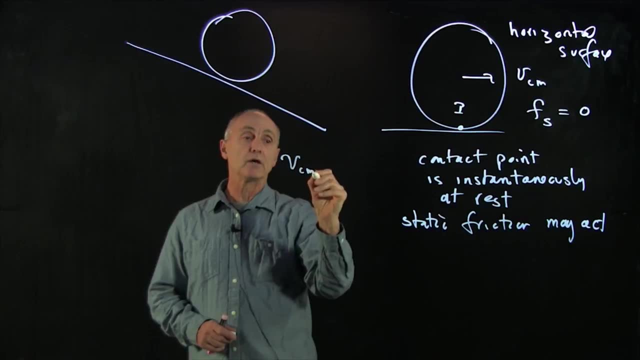 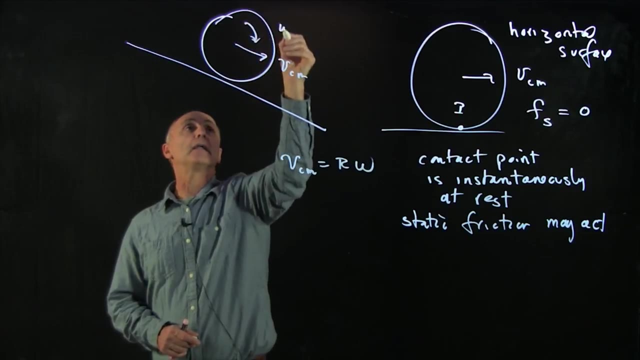 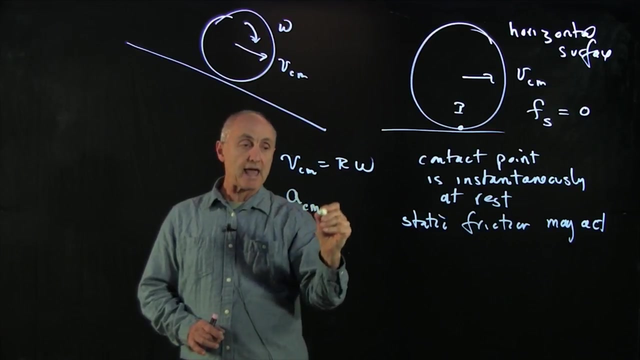 wheel in a vacuum, it will keep on rolling. If a wheel is going down an inclined plane and it wants to maintain the rolling without slipping condition. so here we have VCM and it has some angular speed. we have to be careful because in this case, if we differentiate, ACM is r alpha, So what is making the wheel? 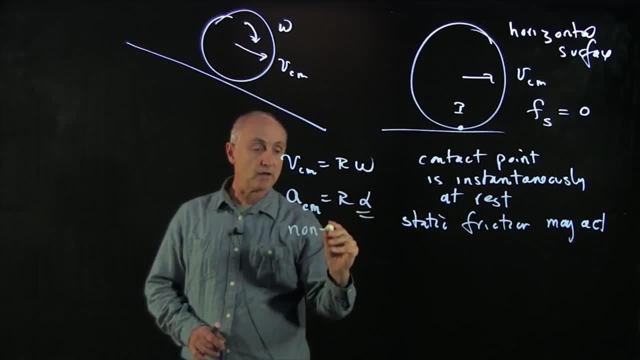 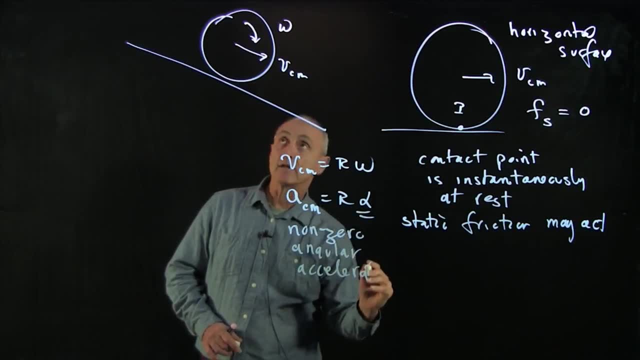 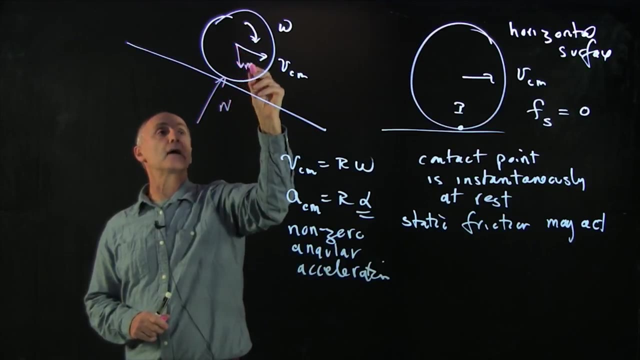 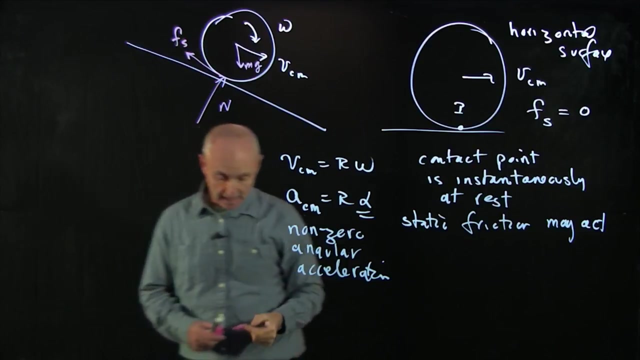 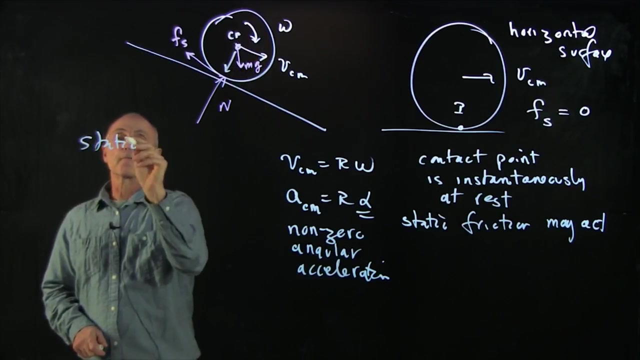 spin faster. It has a non-zero spin, And if we look at the forces acting on the wheel, then we have a normal force, we have gravity acting at the center of mass and we also have static friction, And it's precisely the static friction that is producing the wheel. 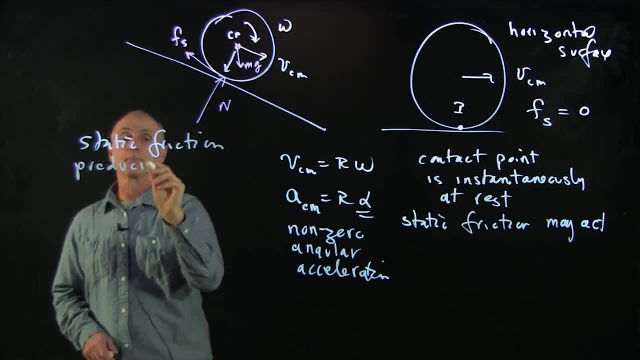 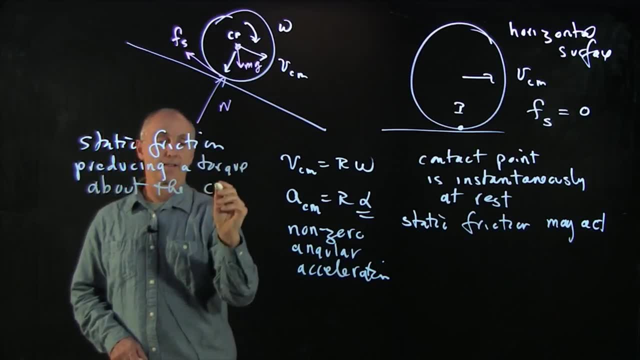 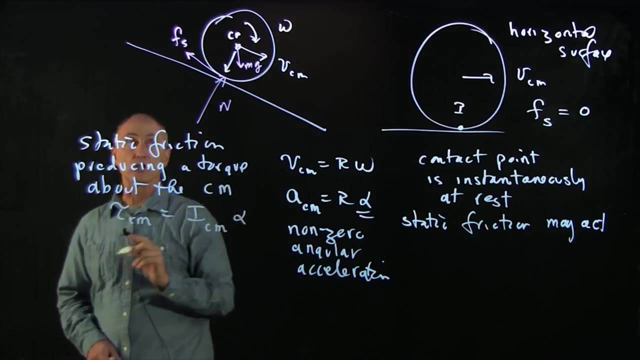 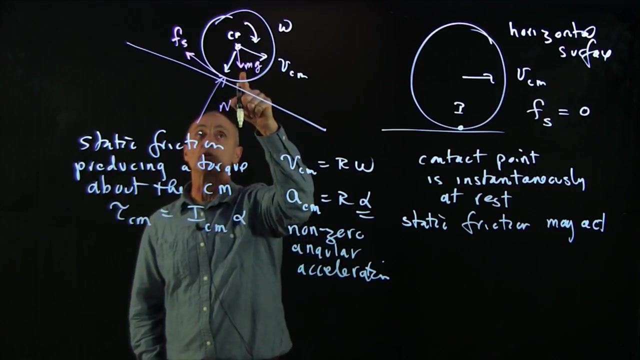 So if the car-wheel shifts, we get the same thing. it's just the force acting on the wheel, But it's also the center of mass And when the car-wheel is purchase, it has the same force acting. So if the car-wheel is actually Laminar and then it's resting on the wheel, overall it's. 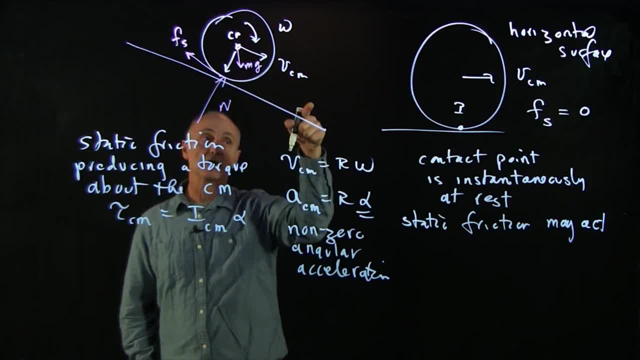 making a torque about the center of mass, And that torque about the center of mass will produce an angular acceleration. So in order for the wheel to continue rolling without slipping, it must have both a linear acceleration, which comes from gravitational force component going down the inclined plane, minus one minus one, minus two, minus three, minus ten minus 14..